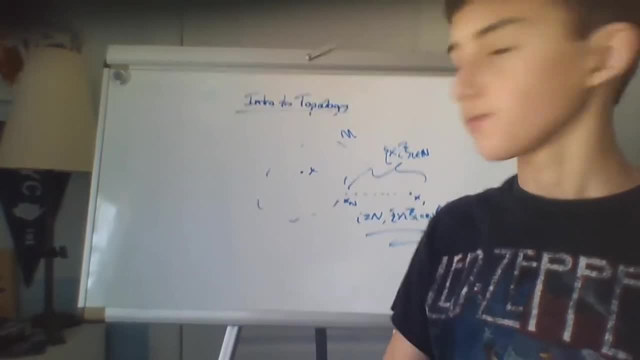 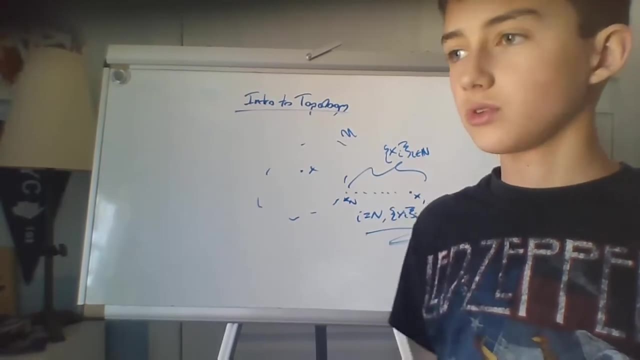 the notion of convergence in this way, with open sets, okay, or with neighborhoods. So what I want to address next is what's going to happen when we have a neighborhood that's sufficiently close to x, What desirable properties should, if we were to define a collection of open sets on a collection of? 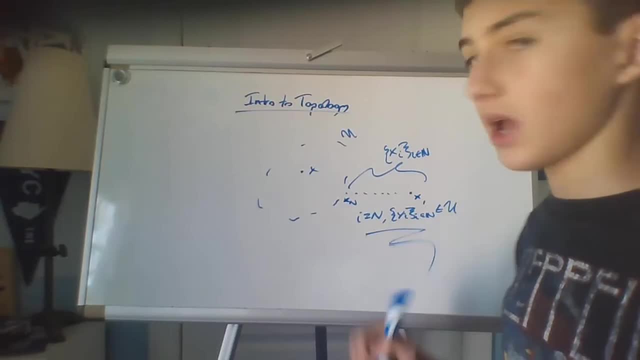 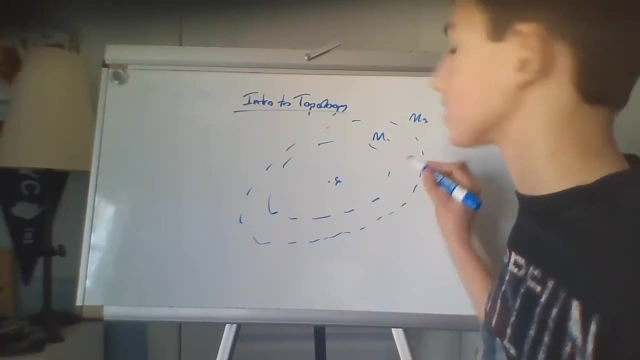 sets which satisfy a specific criterion, then what should we have that criterion be? So again, I've got my point x, but this time I've got two open neighborhoods, one of which contains the other around x, And what I want to address first is: should this collection of open sets be closed? 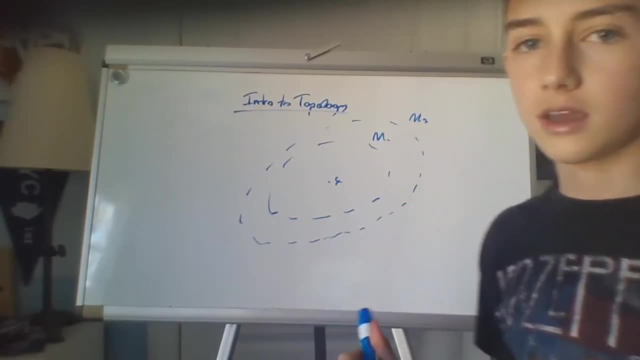 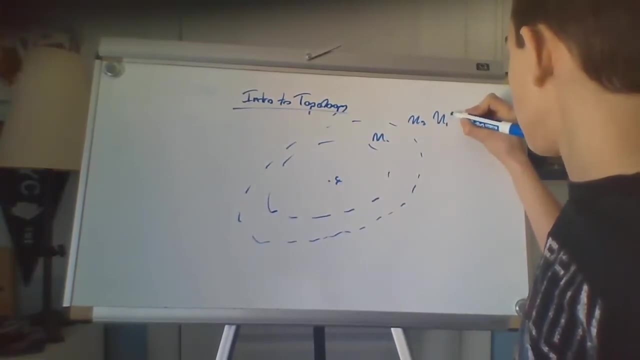 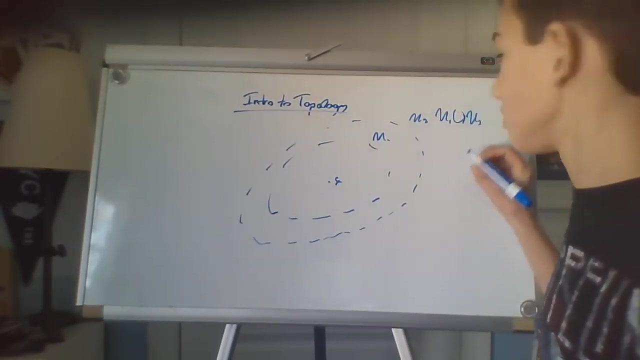 under union And, if so, what kind of union: Finite union, countable union or arbitrary union? even So, basically, what we want to address is: is u1 union, u2 open? Well, this is an easy question to answer, because u2 union, u1, obviously, since u2 contains u1, is going to be u2,. 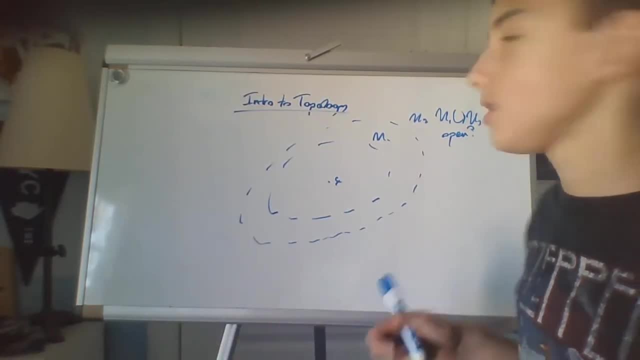 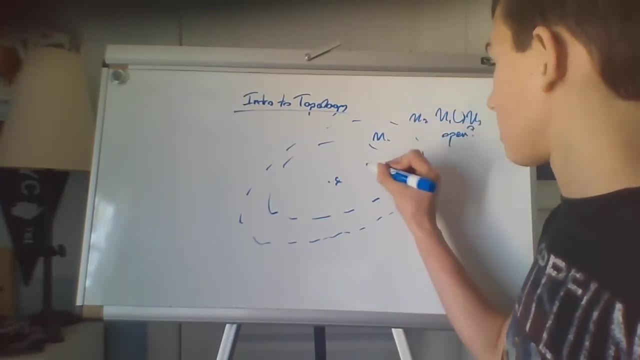 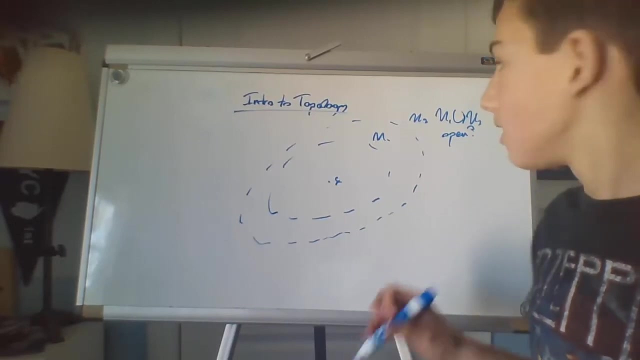 and u2 is an open set, so hence we've proven our condition. So it is indeed closed under union. If we moved u2 into here and had, uh, countably or even infinitely many, arbitrarily many um elements in this sequence, then it's still going to be an open neighborhood because there 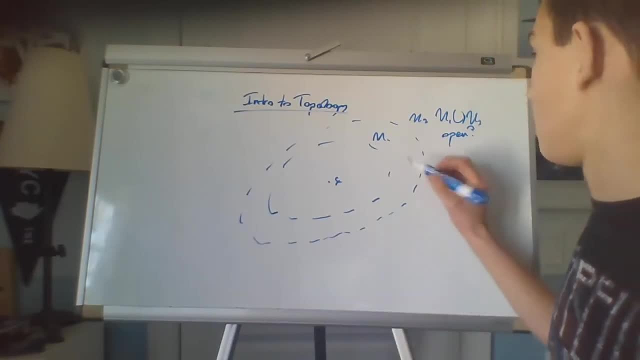 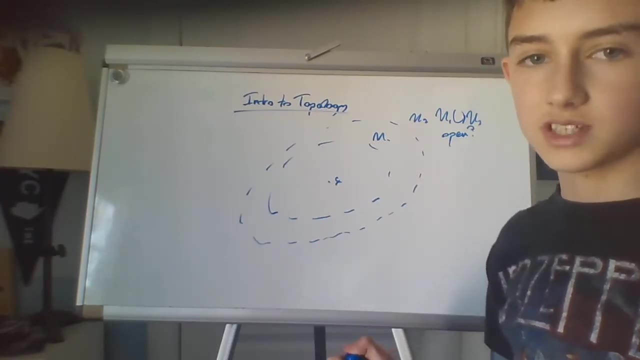 still has to be a biggest neighborhood. no matter, uh, there still has to be a biggest neighborhood. And even if they were equal to each other, if they were all equal to each other, similarly, the union of something with itself, over and over again, is just itself. 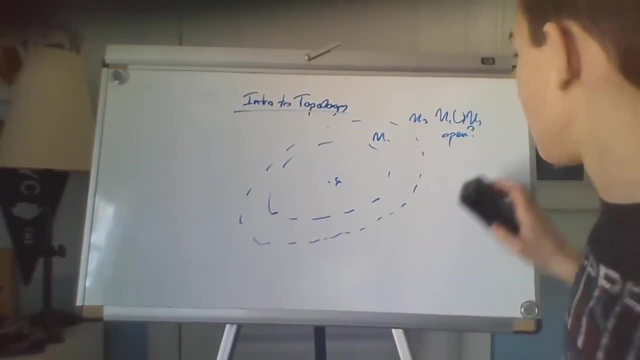 So hence we can say that it's closed under arbitrary union. It doesn't matter if it's finitely many values in the sequence or infinitely many. So hence we can conclude that it's closed under arbitrary union. So now to address intersection. 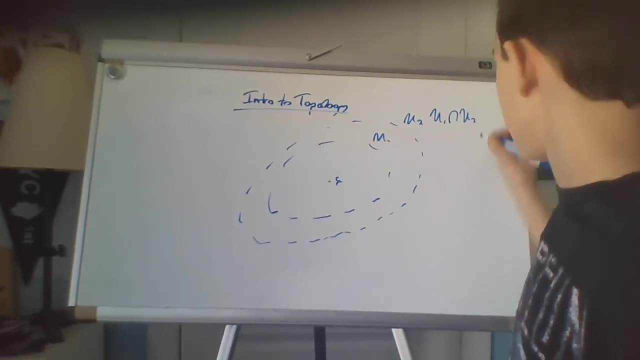 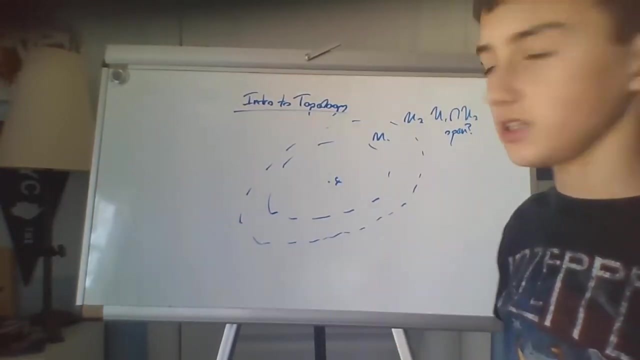 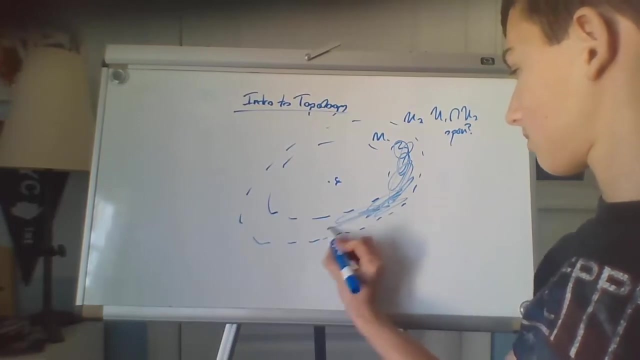 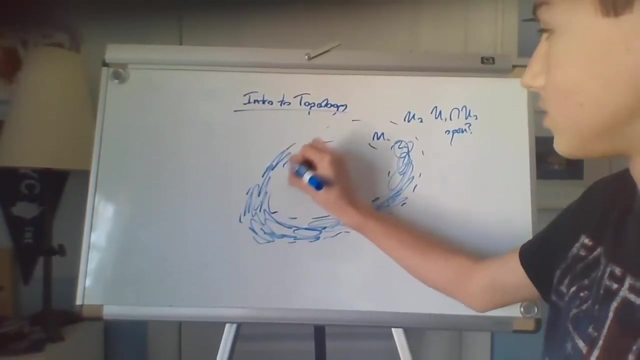 So the question now is: you intersect U2 open Now, once again, this is easy if we have countably many. So this shaded area here is going to be the area in question, And of course, this should be. 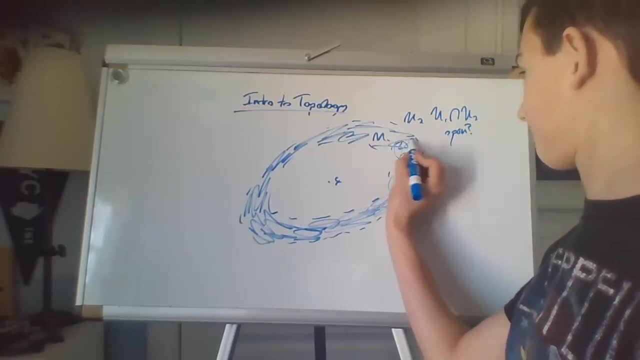 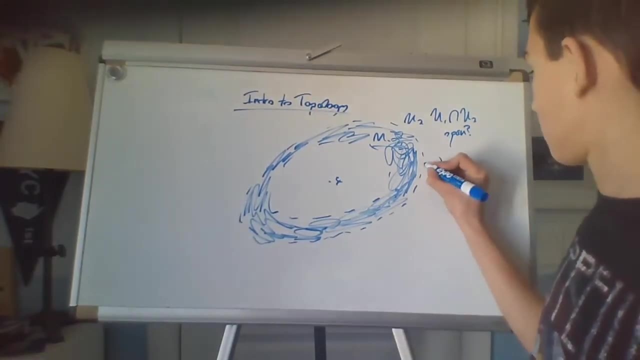 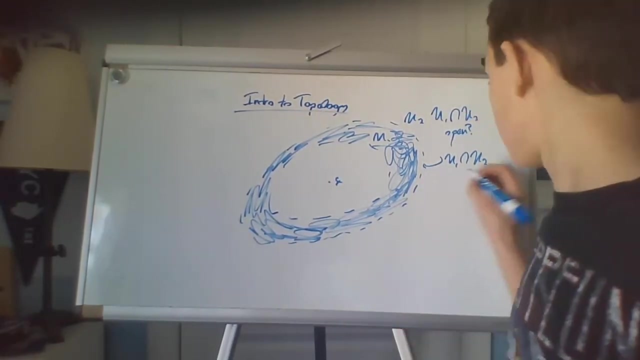 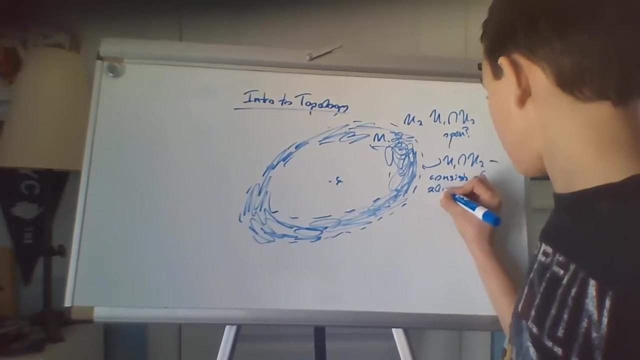 Well, we don't know that yet, but So this blue shaded area is U1, intersect U2.. And well, what does this consist of? fundamentally Consists of all. Well, what is U1?? It consists of what's in U1 and U2.. 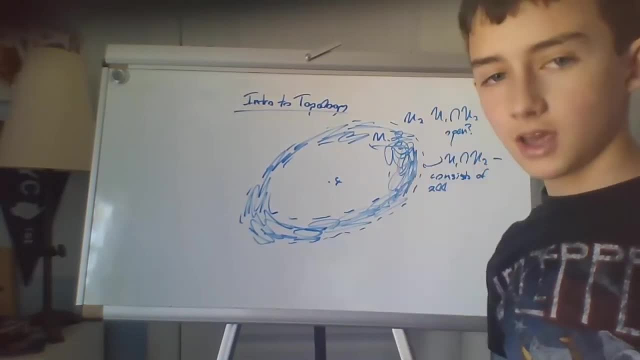 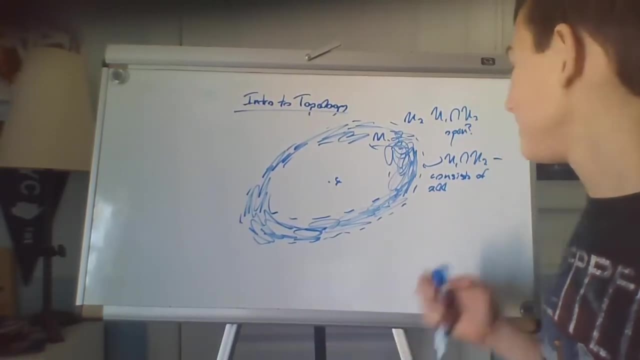 But what's in U1?? It's all the values that are sufficiently close to X according to U1, or U1 sufficiently close to X, And similarly, In a similar way, for U2.. So, basically, it's all the points that are sufficiently close to X. 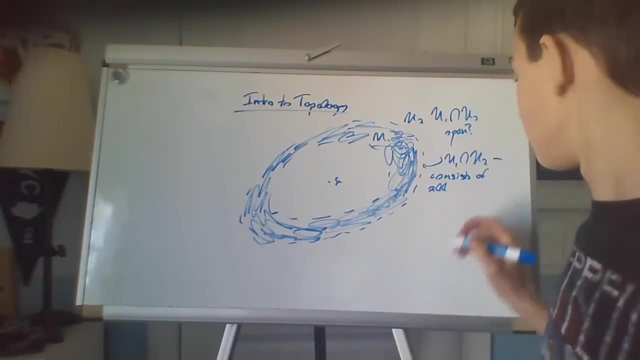 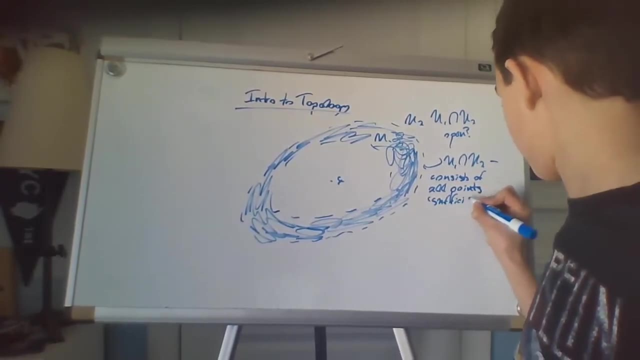 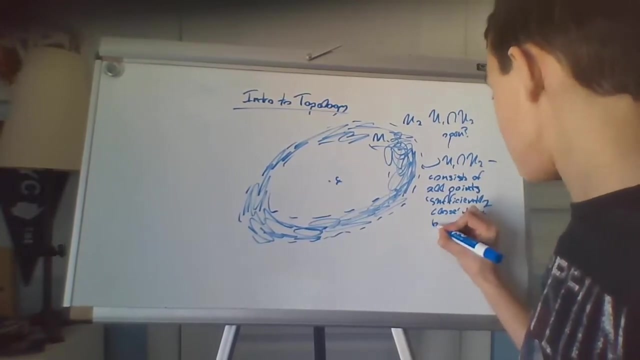 by the nomenclature of U1 and U2.. So it consists of all points sufficiently close to X by the nomenclature of U1 and U2.. So it's this shaded area here, But it doesn't matter what the nomenclature is. 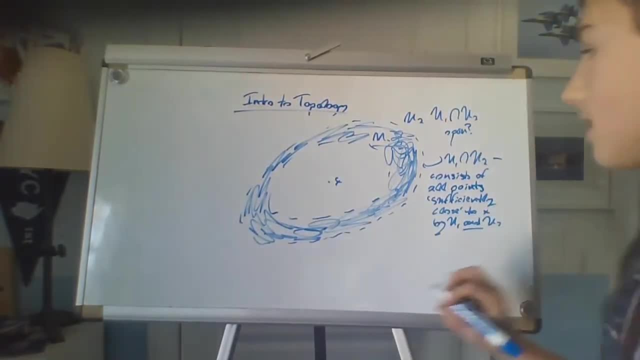 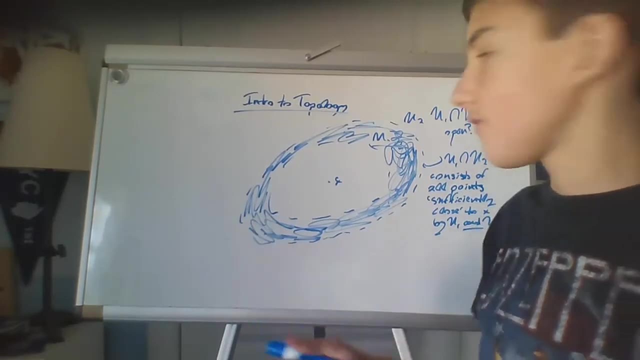 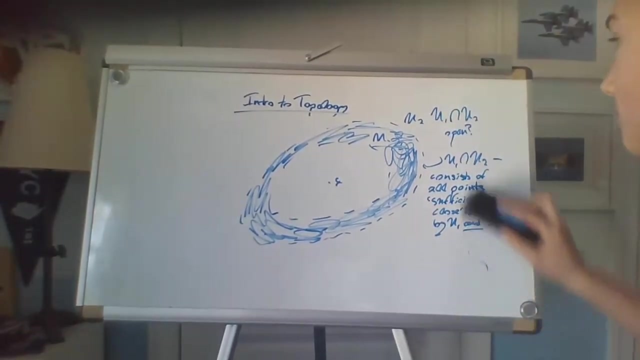 It's still sufficiently close, in a way. So hence we can conclude that for countably many of these, for a final, finitely many of these, it's closed under this operation. But here is where the problem arises. 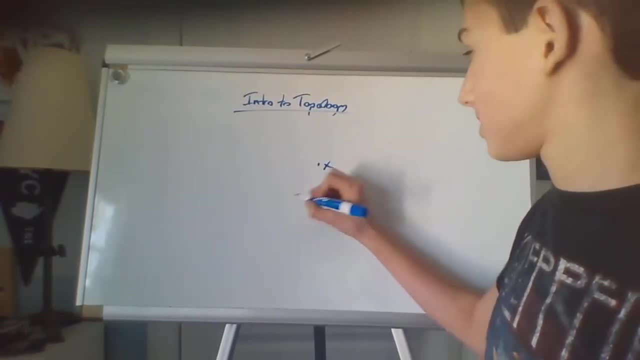 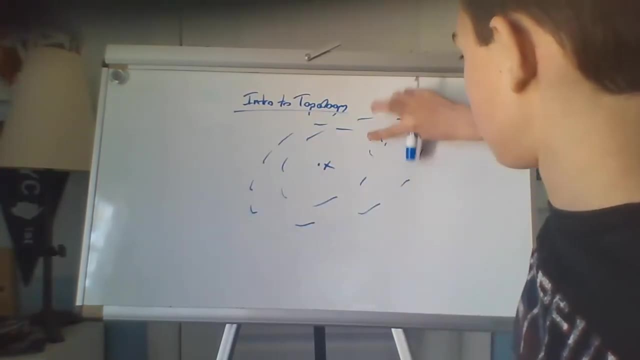 So, once again, X, U1, and well, here I'll make this a little better. I'll make this U1,, this U2, and then you know, all the way on to U infinity. So we've got a sequence now. 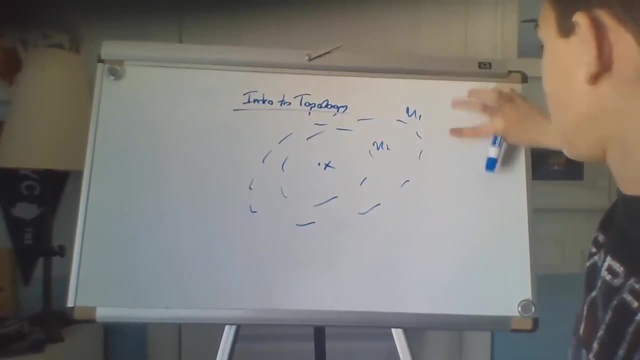 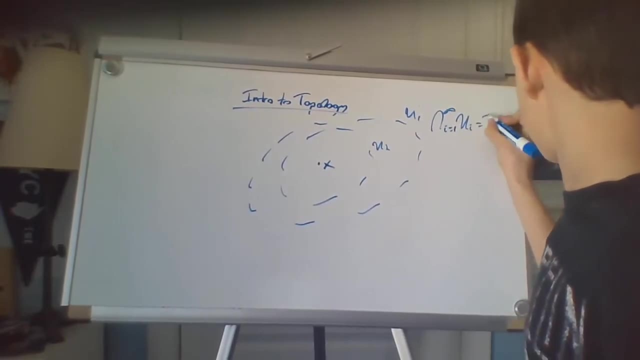 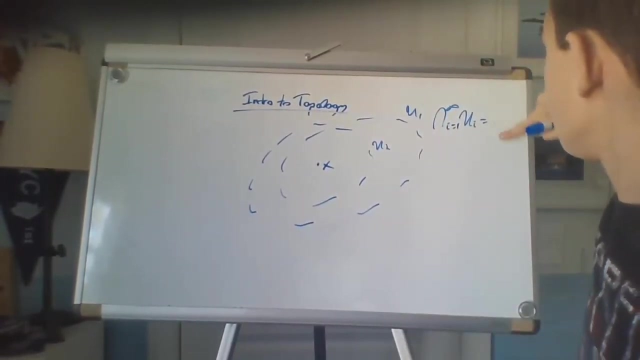 an infinite sequence of these. But if we take their intersection over all I, what's that going to be? Well, once we get smaller and smaller, it's going to get infinitely close to X. So, of course, the intersection over all of this. 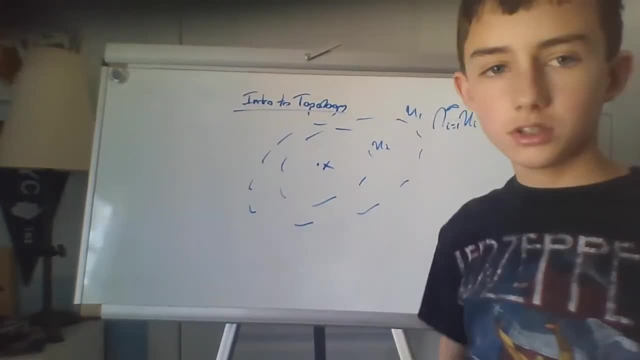 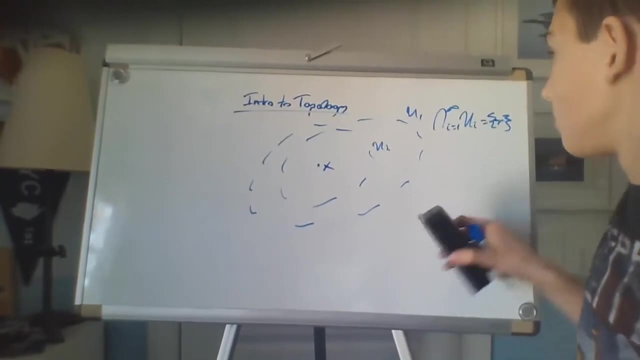 is going to be X And because it excludes everything. this isn't an open interval. It's an infinitely small open interval, but we can't really have that. So to make this more concrete, allow me to show you another example of this. 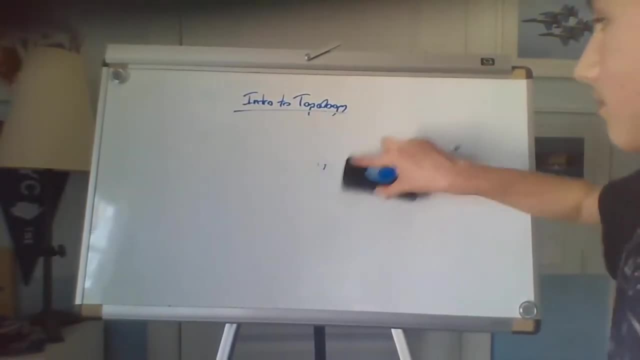 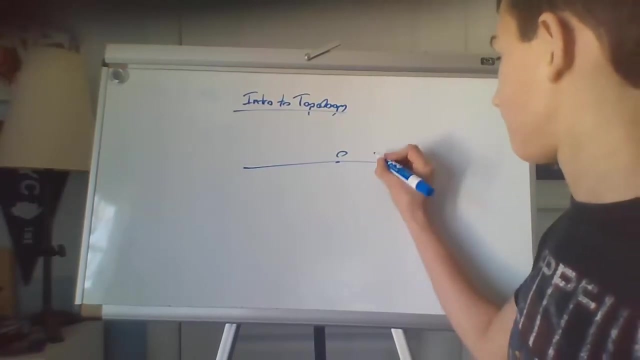 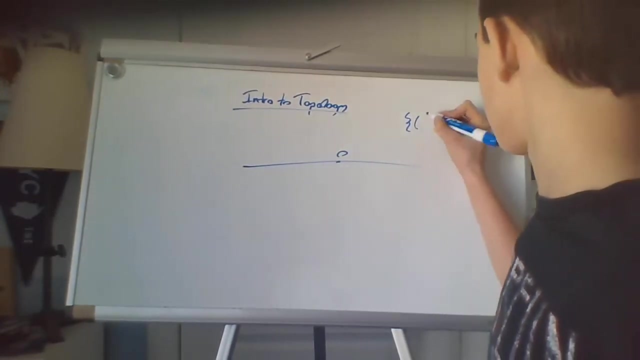 So I'll take the real line centered at zero Zero. So take the sequence of intervals of um one minus one over two, Minus one over n, to n Um n in the natural numbers. Let's take this sequence. 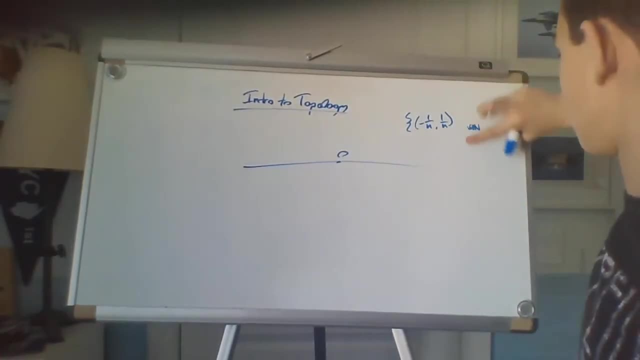 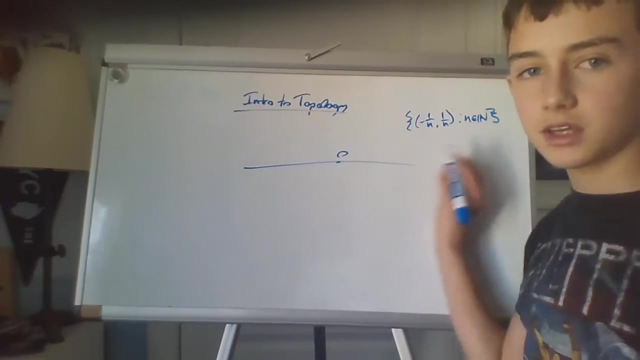 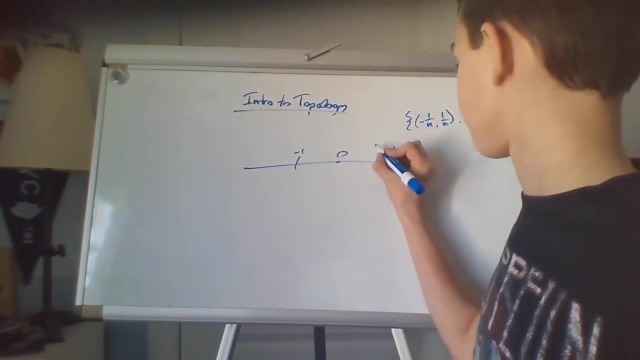 Um, or here is probably a little better way to write this, So let's take this sequence here And okay, we'll start out at one. So one negative one, Um, one, two, One minus one, two. 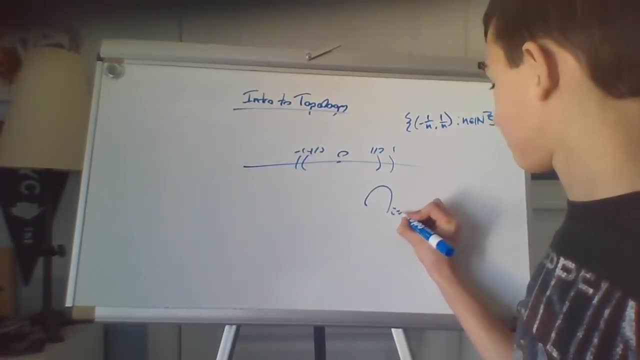 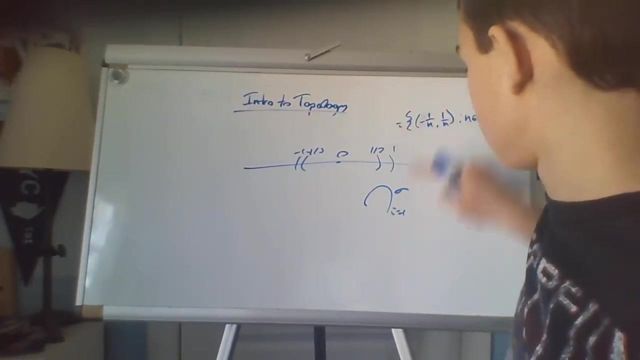 And so on, And taking their intersection. once again, we're left with the center of all of these. So, um, I'll just call this uh. I'll call this the I. Uh, that's not a good idea. 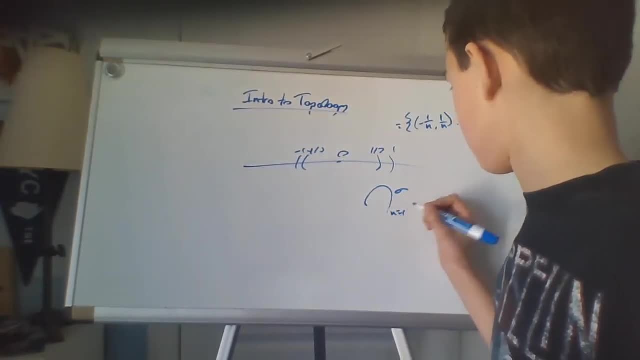 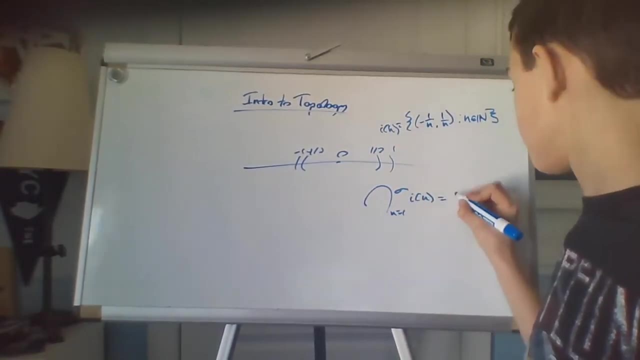 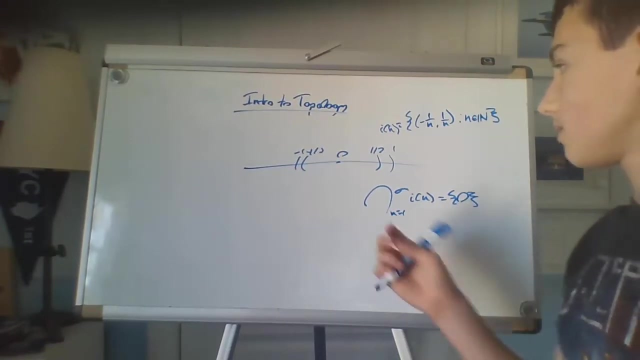 Well, actually it is, but I just used the wrong index Um. I'll call this I of n, I of n. Once again, this is set um containing zero Right, Just the one element. set zero For a similar reason. 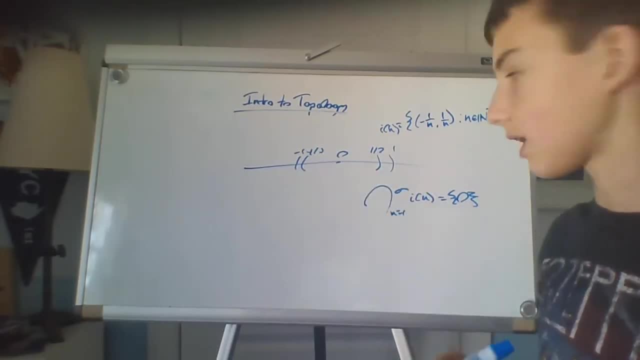 it's going to get infinitely small and then, once we take their intersection, it's all going to go back to zero, right? We could do the same thing for balls or, uh, hyperspheres or whatever you wanted to do, right? 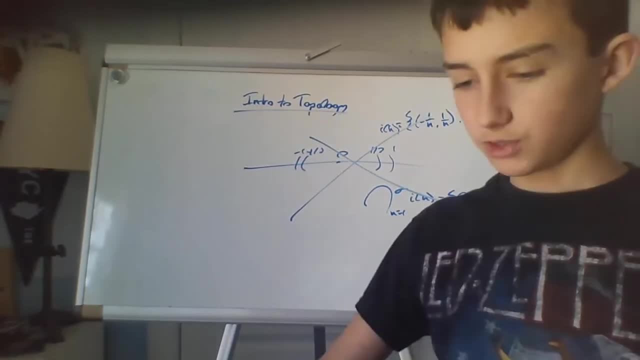 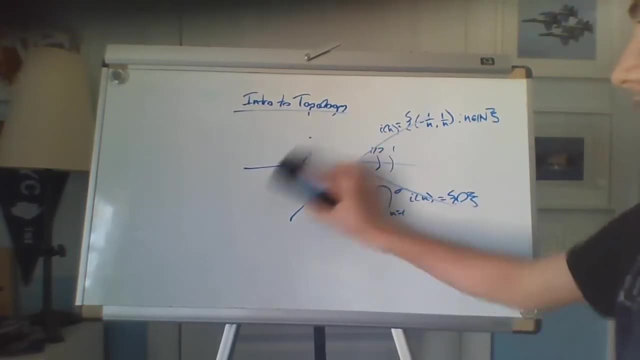 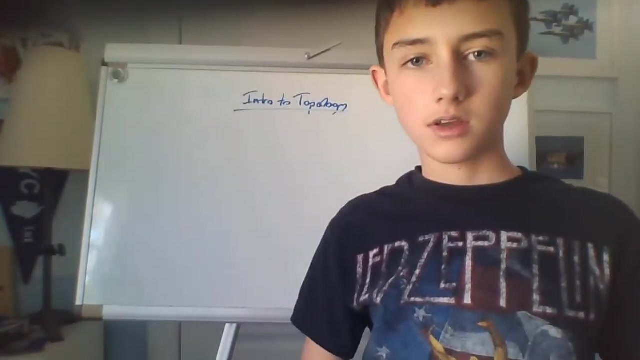 This is a huge no-no, As we have shown twice. Whoa, Um, so um. hence, now we have all of the desirable properties that we need to define this alleged collection of open neighborhoods. So what we call this is its apology. 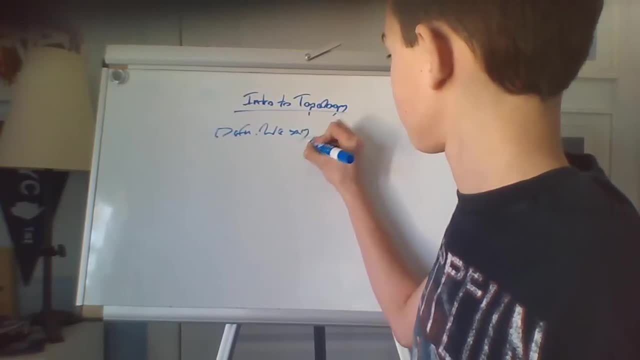 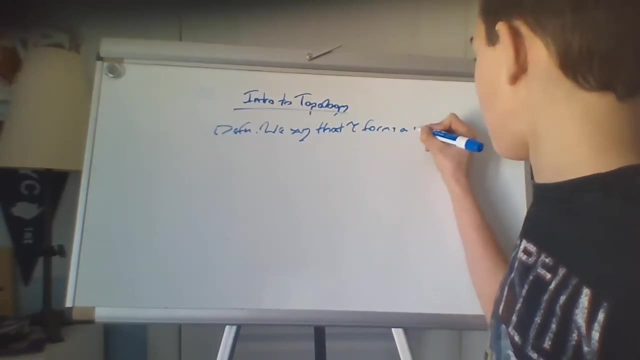 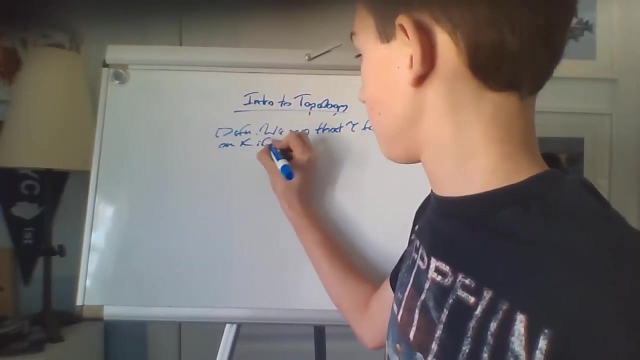 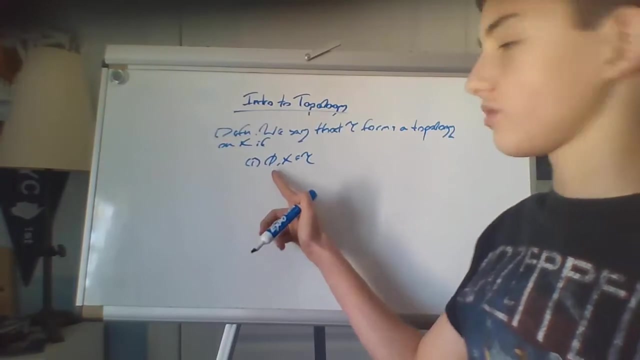 So we say that tau forms its apology on x, if one the empty set and x are in tau. So we're just setting uh. first of all, we're setting um, an infimum for what we want the topology to be. 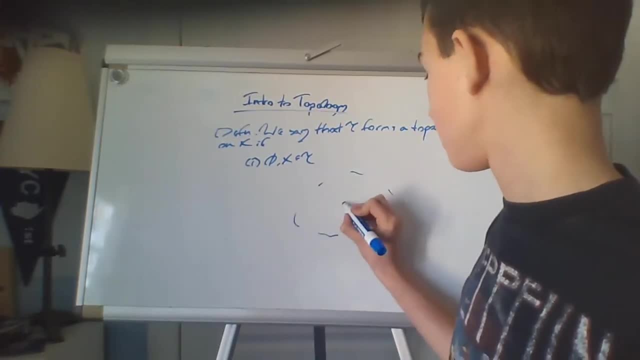 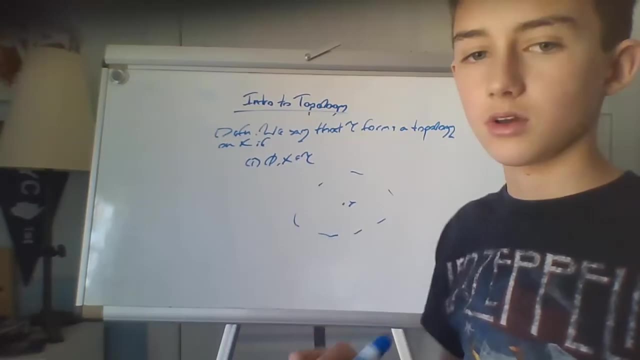 and here it has to contain x, because of course all of the open intervals contain x. and then we take the union of all of these Collectively, all of these points are x, and if all of them contain all of the x's individually, 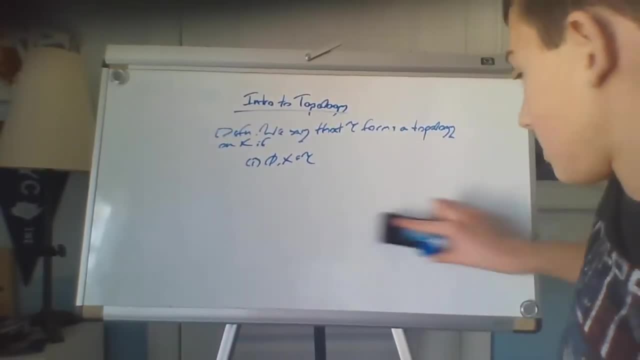 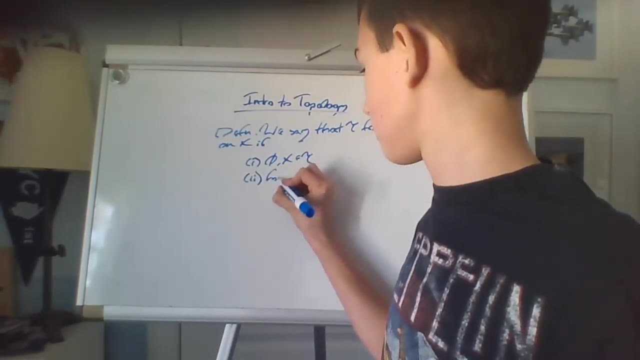 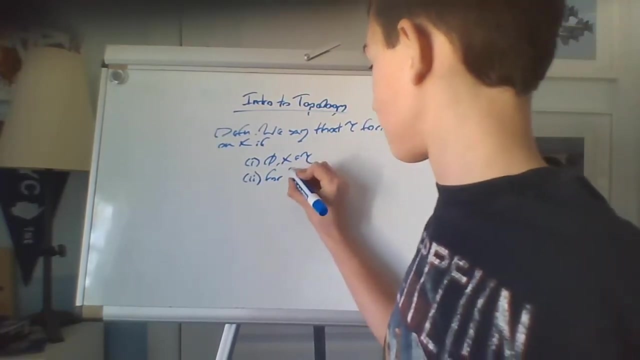 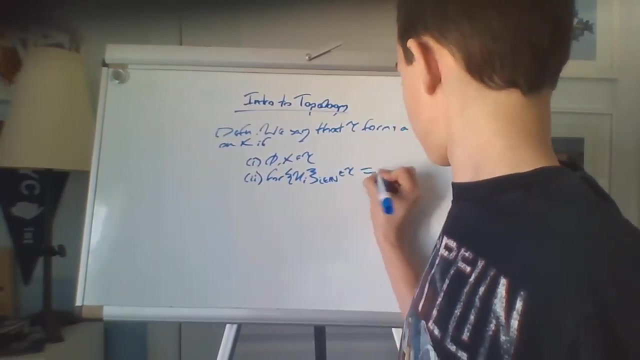 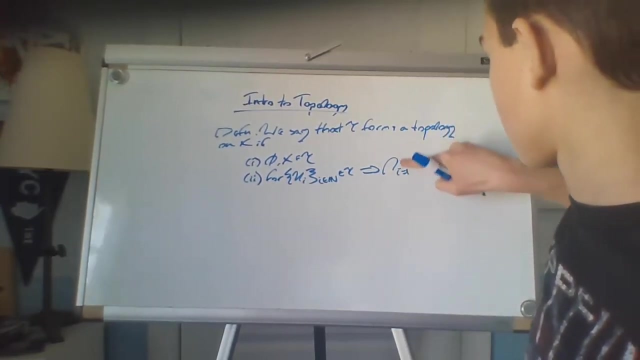 x has to be an element of tau Right Now, the two properties we discussed: um for some sequence u of i, some sequence u of i, um in tau, um in tau, um, their intersection um, their intersection, their um, um accountable. 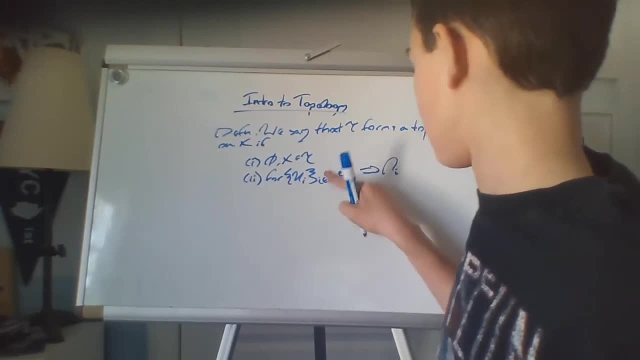 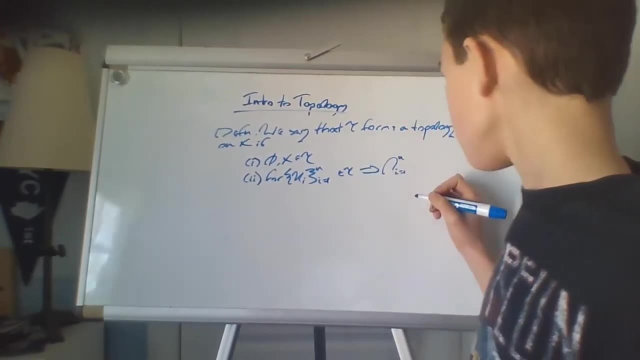 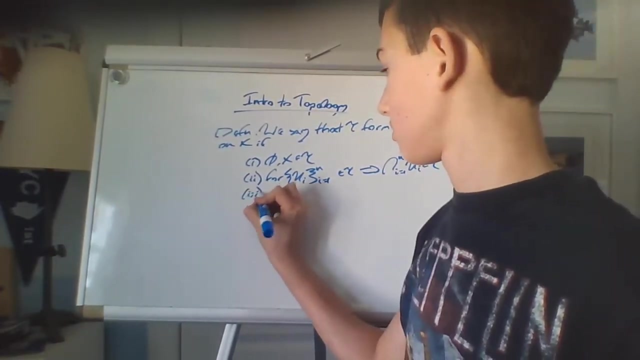 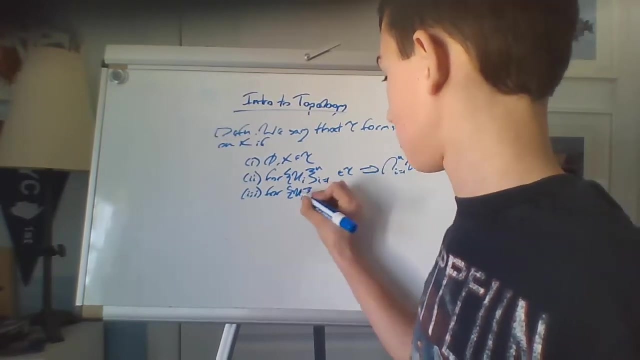 um, here I should. I should write this better, because it's not all natural numbers. natural numbers, Uh, all the UIs. a collection of sets is in tau, as we showed, so motivated, at least. so for UI, I should write this better: u, alpha, alpha and a, so 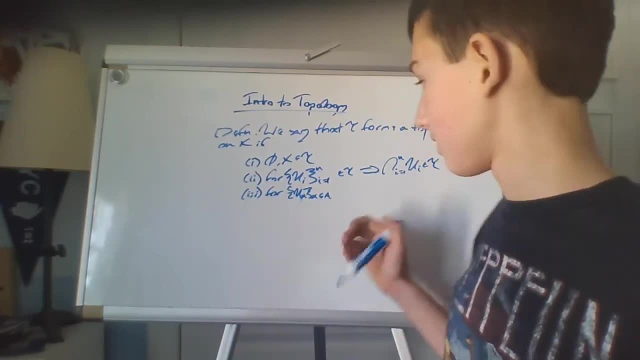 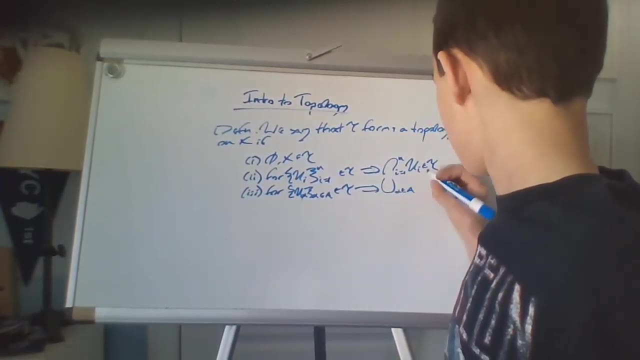 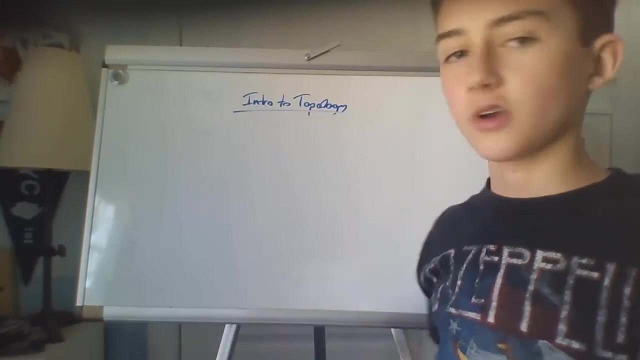 we're just using a as a placeholder- could be infinite or finite in tau, then union of alpha and a of all the u alphas is in tau. so now, as I previously motivated, let's um see how we can define formally the notion of convergence on a. 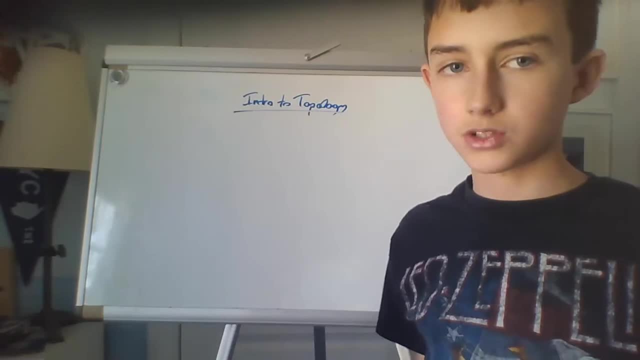 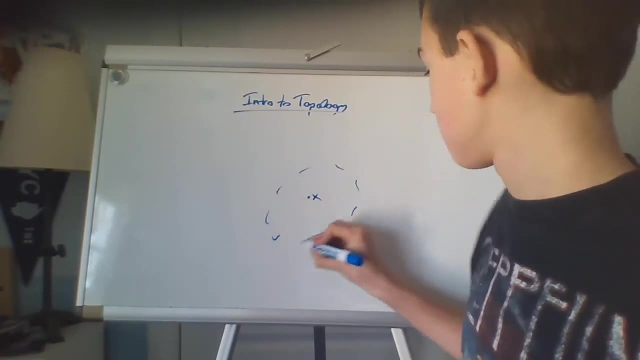 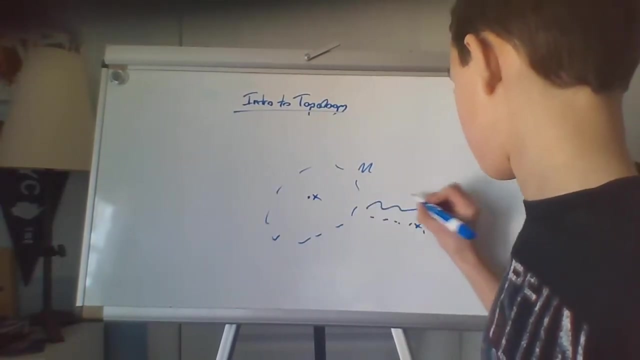 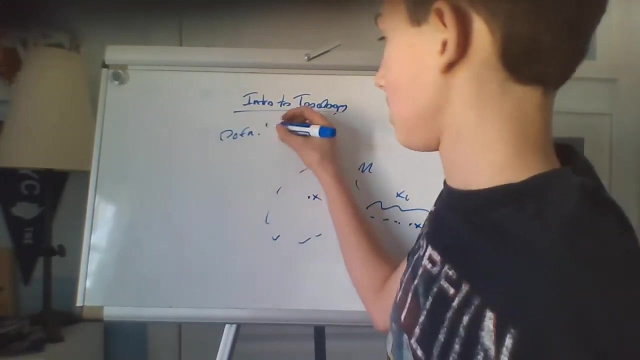 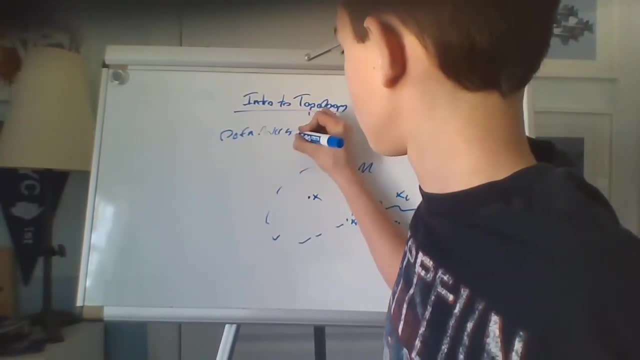 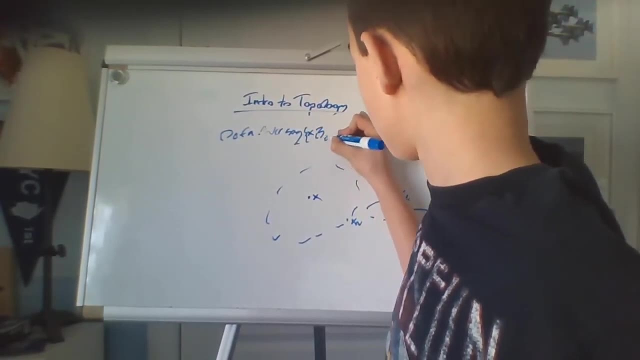 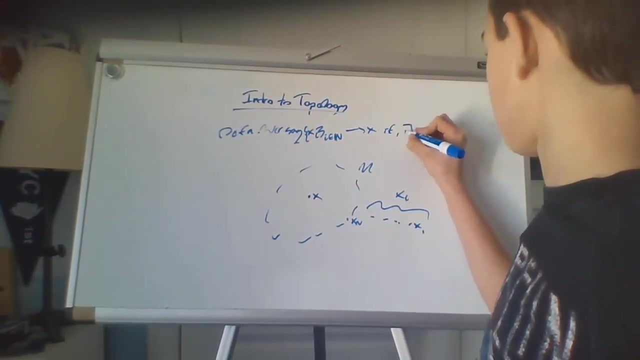 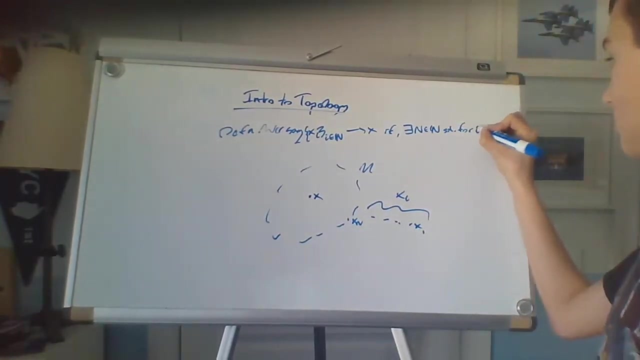 X, n. so no definition should be X, n, so no definition should be. we say X, I. a sequence of points, natural numbers, converges to point X if there exists an N in the natural numbers such that for I greater than n, X, n is. there exists an N in the natural numbers such that for I greater than n, X, n is. 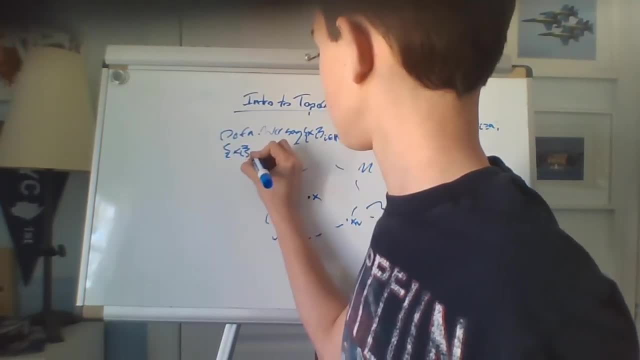 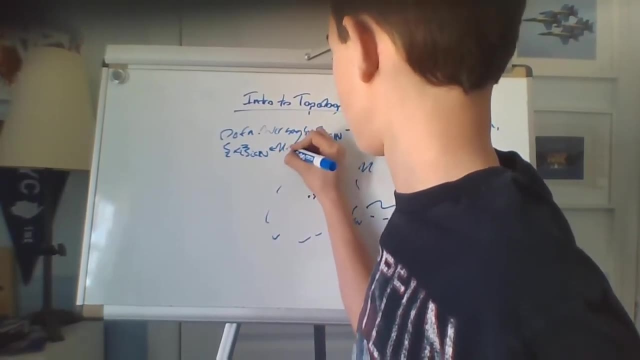 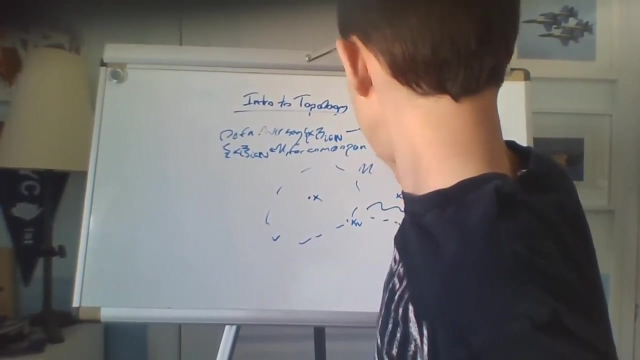 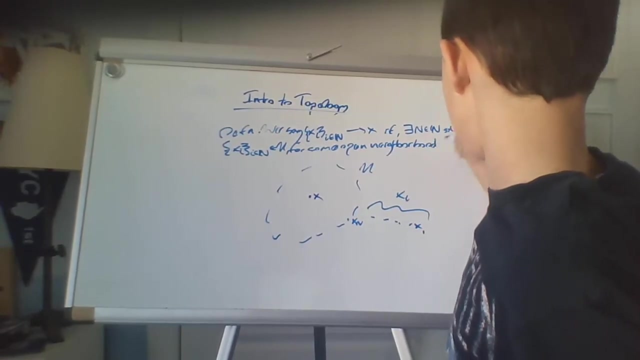 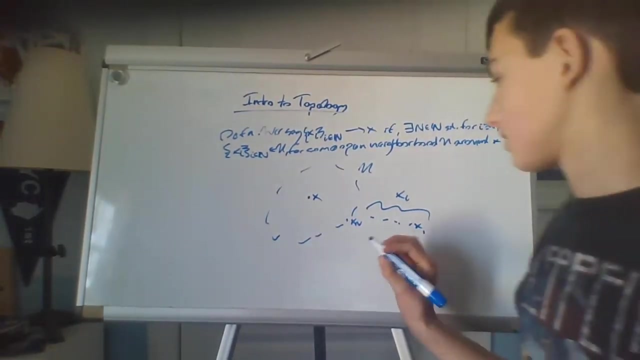 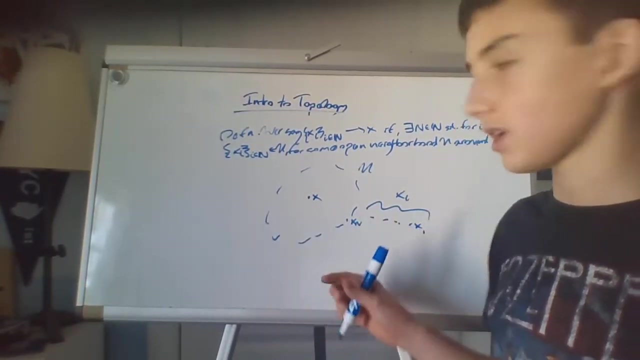 there exists an N in the natural numbers, such that for I, greater than n, X, n is, i is in you for some open neighborhood. hood you around X. hood you around X, hood you around X. so this makes sense. if we make this, the boundary point, sufficiently close to X, then we can make this point sufficiently close to X and then all of them will be inside of that. 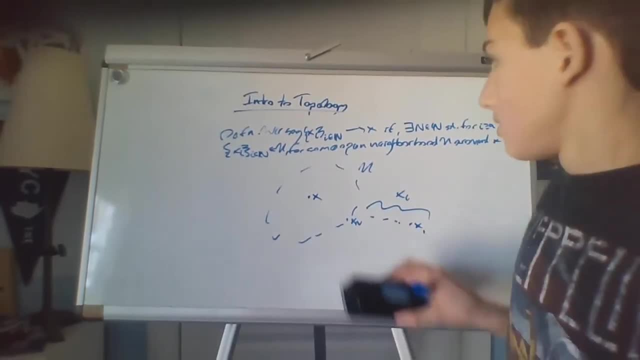 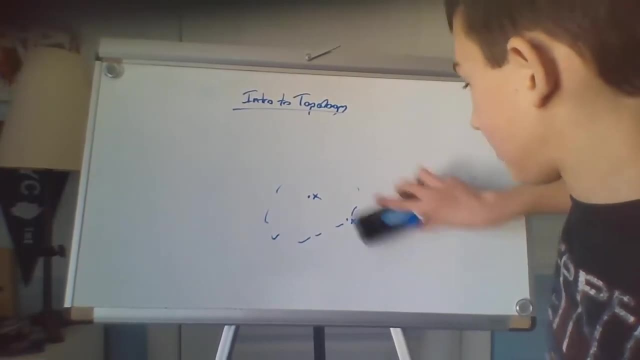 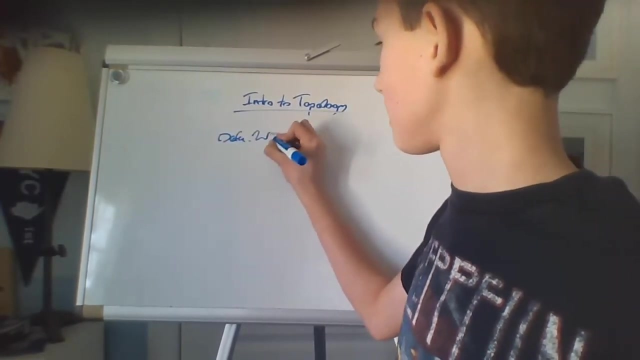 so this is convergence. now what about continuity? I haven't really talked about that at all, so we say: so, this is convergence. now what about continuity? I haven't really talked about that at all, so we say: so, this is convergence. now what about continuity? I haven't really talked about that at all. so we say: 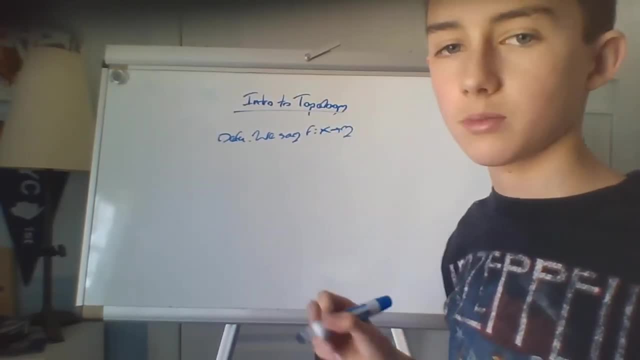 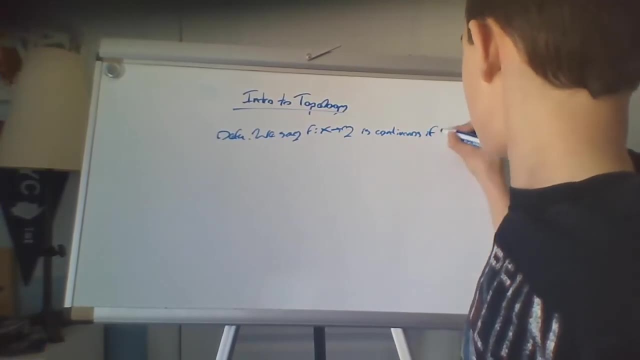 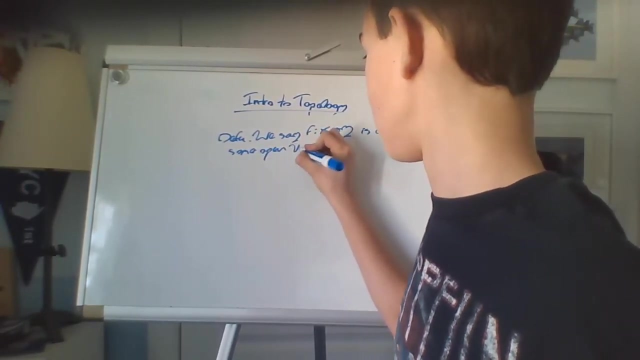 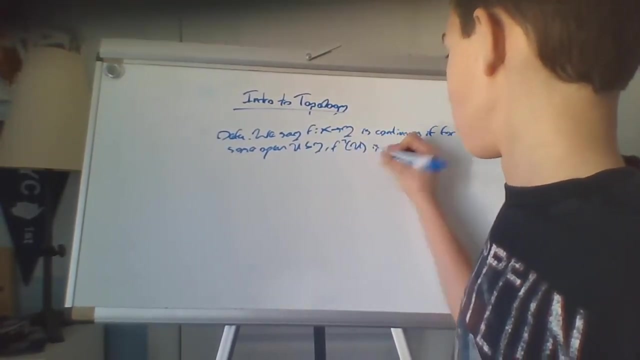